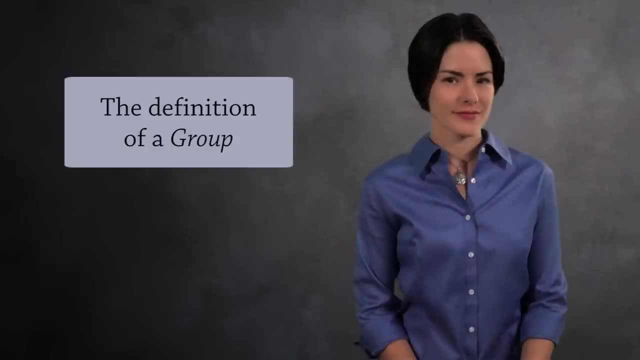 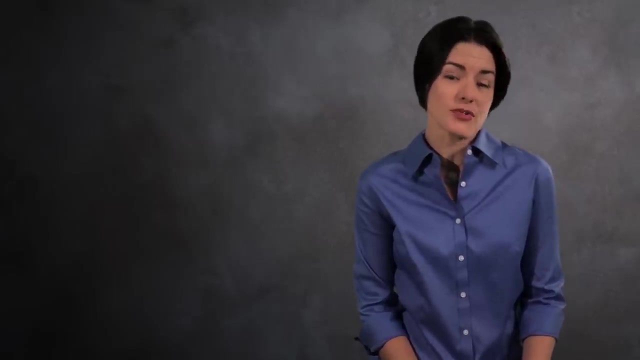 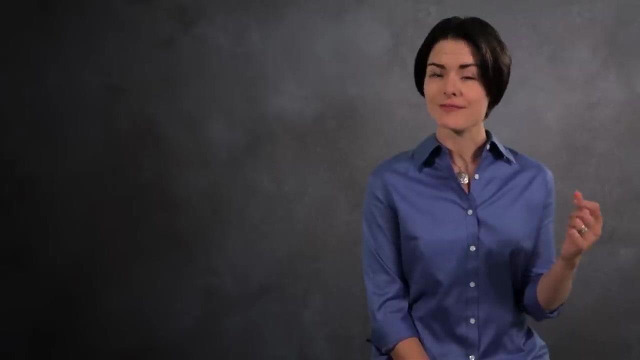 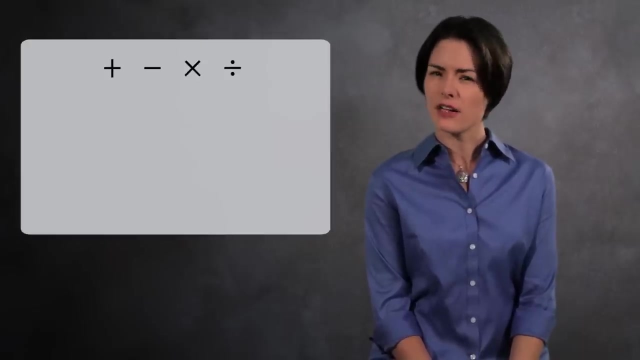 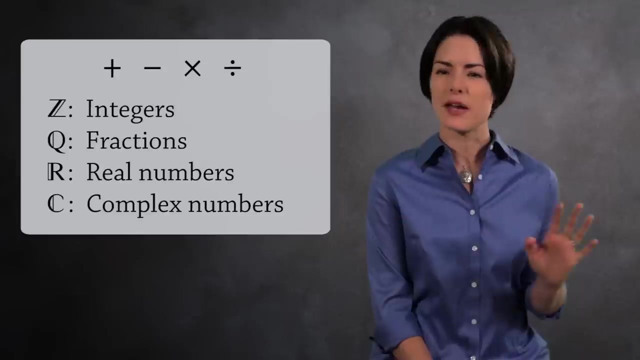 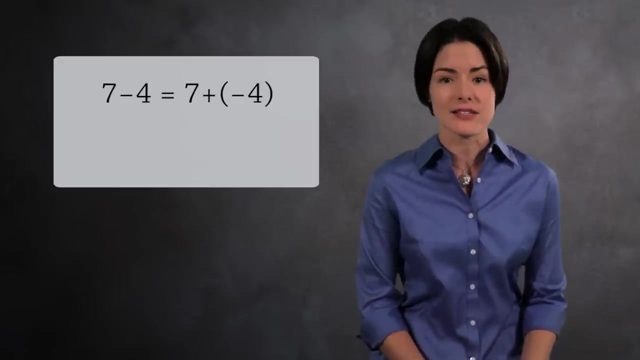 The first time you hear the definition of group, you may think to yourself, it's an abstract idea. But what do you expect from abstract algebra? Because groups are abstract, they generalize a lot of different things from arithmetic, algebra, geometry, and more. This generality is what makes groups so powerful. The mathematics you learn in abstract algebra can be applied to many, many different subjects. To get things started, let's think back to arithmetic. When studying arithmetic, you learn how to add, subtract, multiply, and divide different kinds of numbers. Integers, fractions, real numbers, complex numbers. Then one day, probably when you least expected it, you learn that subtraction is addition in disguise. For example, 7 minus 4 is the same thing as 7 plus negative 4. So instead of subtracting, you're really adding a negative number. 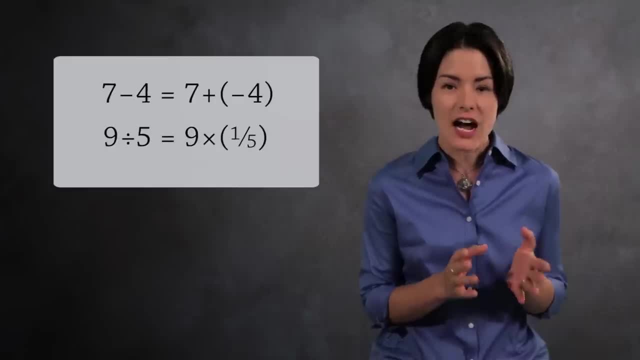 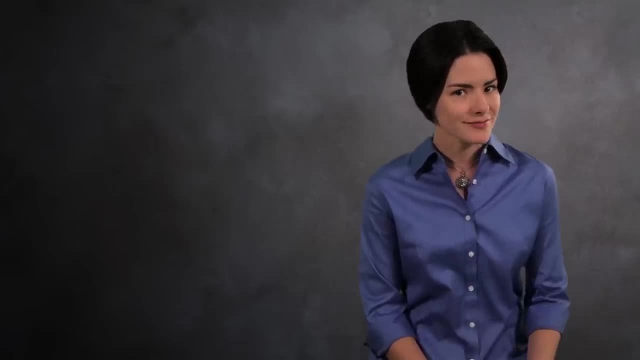 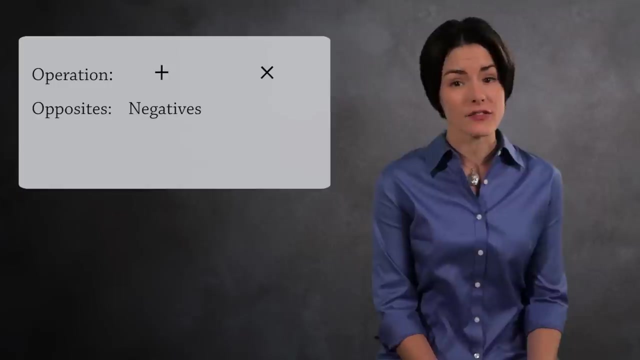 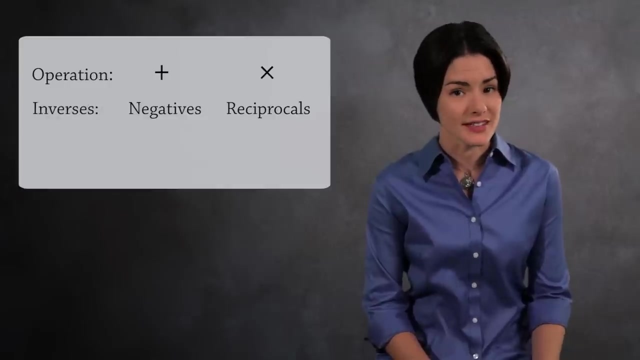 Similarly, is multiplication in disguise. 9 divided by 5 is the same as 9 times 1 5th. Instead of dividing, you're really multiplying by a fraction. So in arithmetic, there are really just two operations, addition and multiplication. For addition, opposites are negative numbers, and for multiplication, opposites are reciprocals. In abstract algebra, we use the word inverse instead of opposite. If you combine a number with its inverse, you get a special number called an identity element. For addition, the identity is 0. If you add 5 and its inverse negative 5, you get 0. What makes 0 unique is if you add it to any number, that number doesn't change. It retains its identity. For multiplication, if you multiply a number by its inverse, it's reciprocal. You get 1. What makes 1 special is if you multiply it by any number, that number does not change. So, for both addition and multiplication, we have numbers.